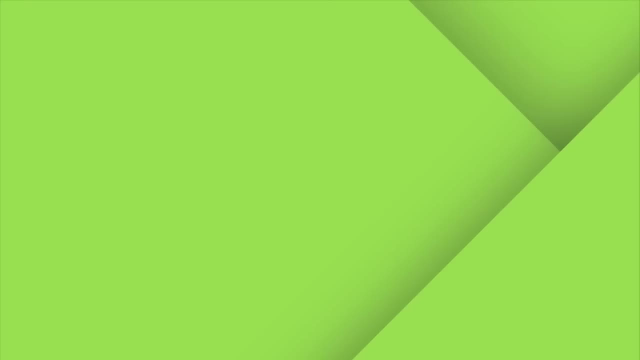 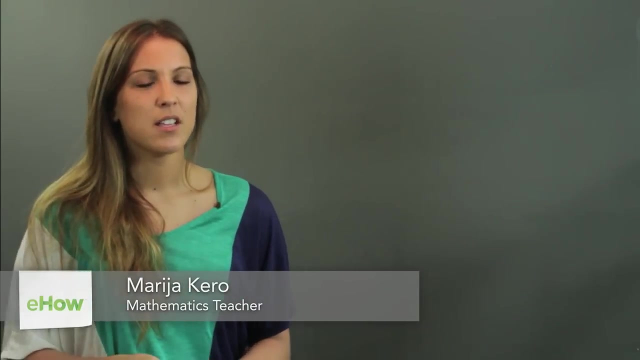 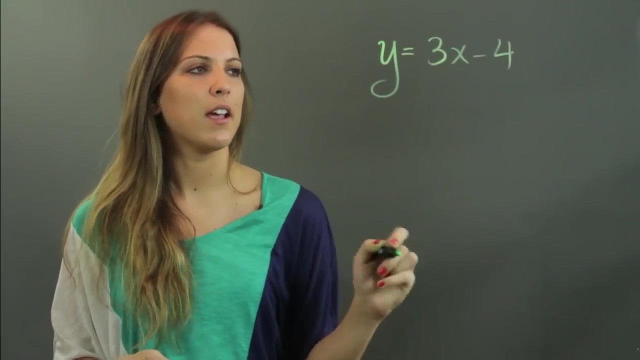 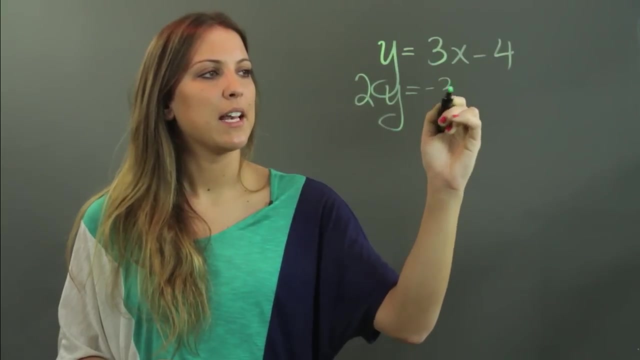 Hi, my name is Maria, I'm a mathematician and I'm going to show you today how to solve linear equations by the elimination method. So if you have a system of linear equations like y equals 3x minus 4, and I have, let's say, 2y equals negative 3x plus 6.. Okay, I 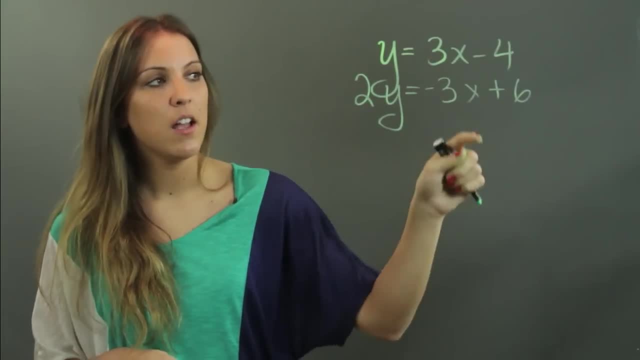 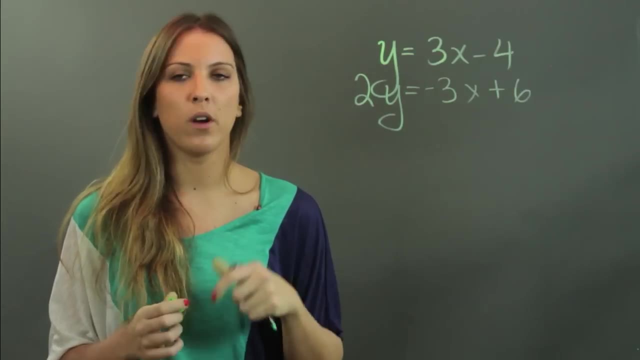 want to use elimination with this specific system because I see that one of my variables has opposite coefficients. So when they have the same or opposite coefficients, you want to use elimination. It's the easiest method, because here's what's going to happen When. 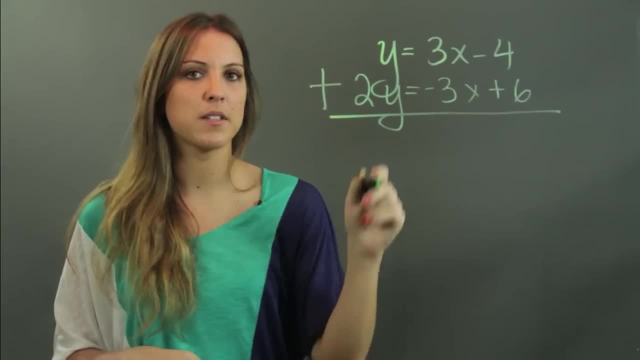 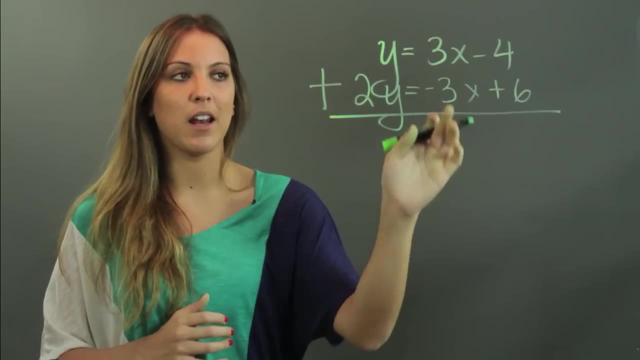 they have opposite coefficients you're going to add. If they would have been the same, I would have subtracted my equations. So what's going to happen is, when I add these two equations, I'm going to eliminate my x variable and I'll be left with just y, which makes it easy. 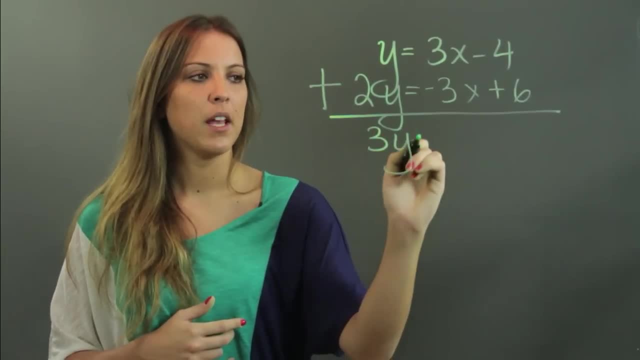 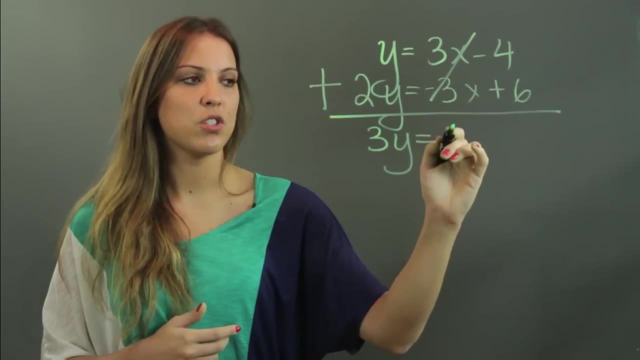 to solve. So I have: y plus 2y is 3y Equals 3x plus negative 3x cancel out. and then I have negative: 4 plus 6 is 2.. And then I'm going to go ahead and solve this equation for y by dividing by 3 on both sides and 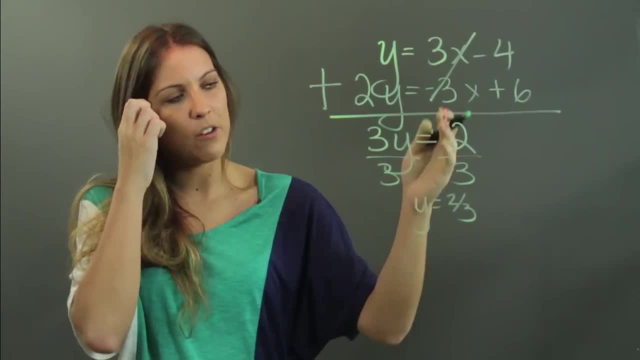 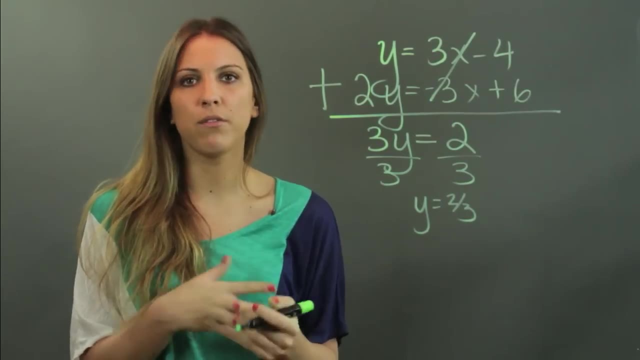 I get y equals 2 thirds. So the whole point of me adding them was to eliminate the x variable so that I'm just left with y, because when an equation is in one variable, then I can solve it. So once you've gotten your y or your x- whichever one you solve for you go. 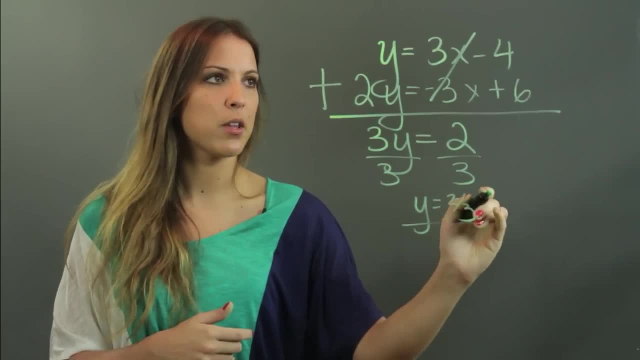 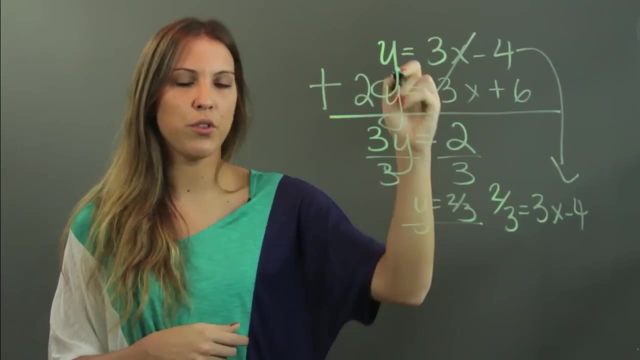 in to get the other value. So if y is 2 thirds, then I'm going to go ahead and write down: 2 thirds equals 3x minus 4.. So I'm rewriting the first equation, but I'm substituting 2. 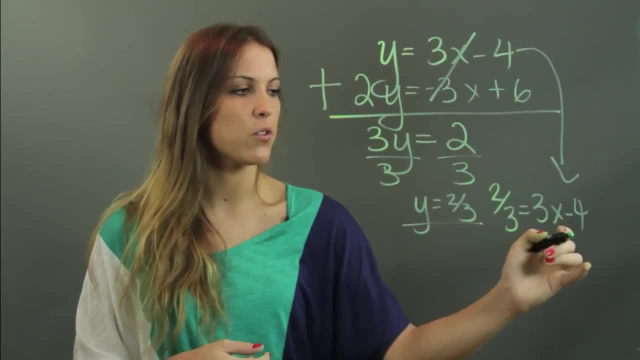 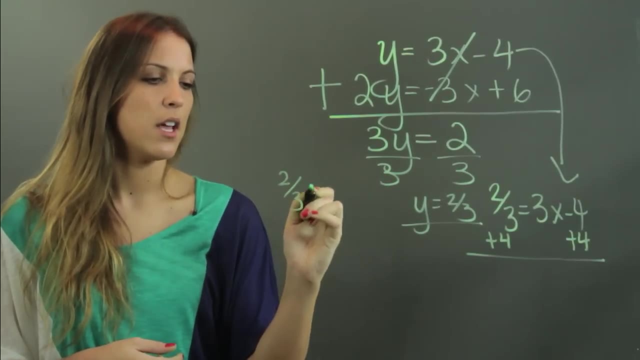 thirds in for y And now I'm going to solve for x. So it's going to be a little sloppy because we have fractions, but we can do it. So we're going to add 4 to both sides. So now I'm doing 2 thirds plus 4, but I know that when I add I have to have the same denominator. 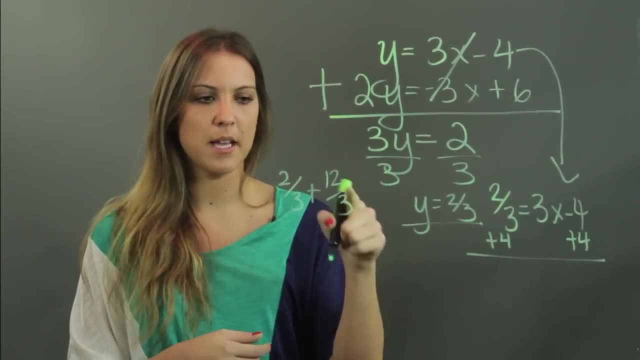 so I'm going to rewrite 4 as 12 over 3, because that's the same thing, right? 12 divided by 3 is 4.. Now that they have the same denominator, I can add them, and that becomes 14 thirds. So